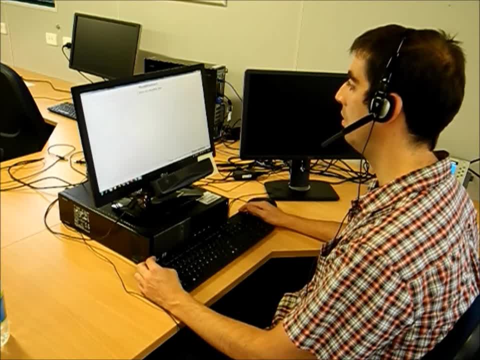 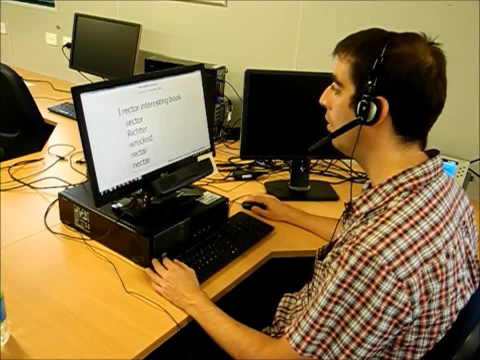 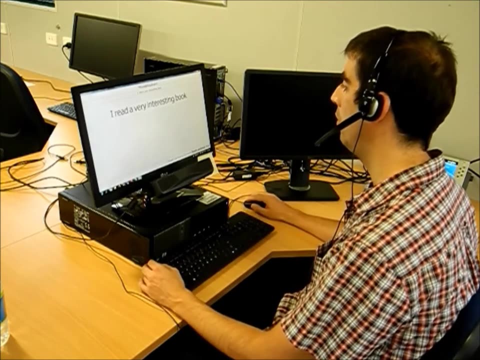 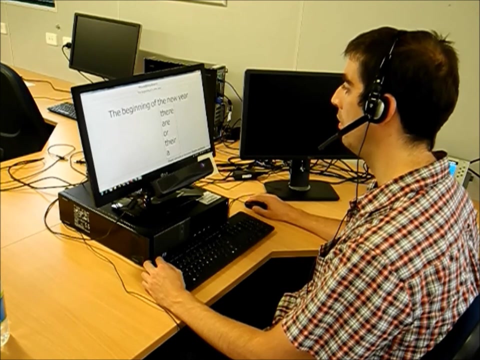 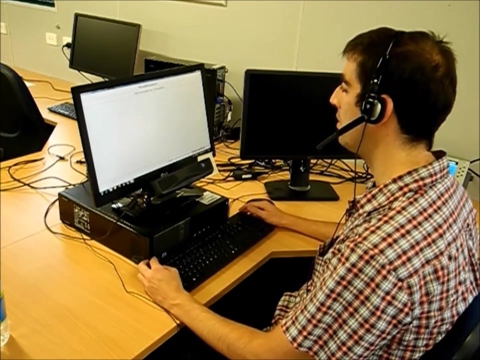 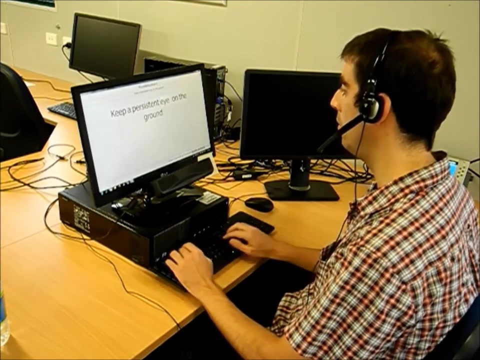 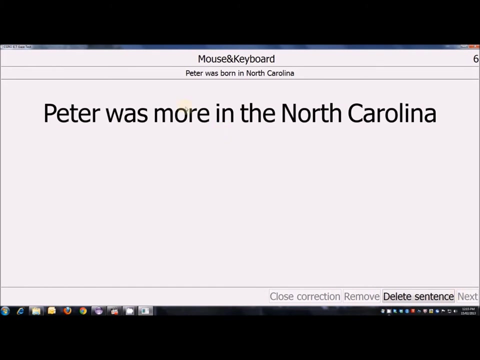 I read a very interesting book. The beginning of a new year. Keep a persistent eye on the ground. Peter was born in North Carolina. Now he lives in aใช merino. He was born in the US. What a beautiful thing. 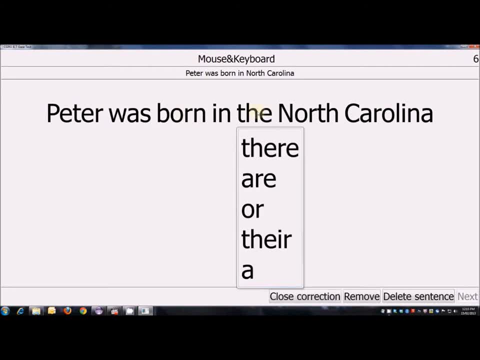 He was born in North Carolina. The whole family lived in the United States. They went abroad. in the United States for the first time The women used their whole families' help by teaching them French. A child with a child, with a child's behavior, was born in Rhode Island. 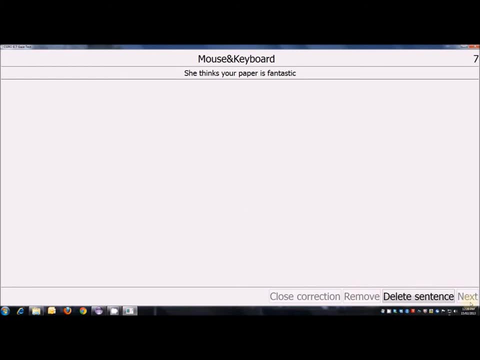 Yes, Wally was born in the United States as well. Yes, Wally was born in The United States as well. He has been in England since then when he grew up. Peter grew up in Ireland. I think he has seen the world, but he never knew the world. 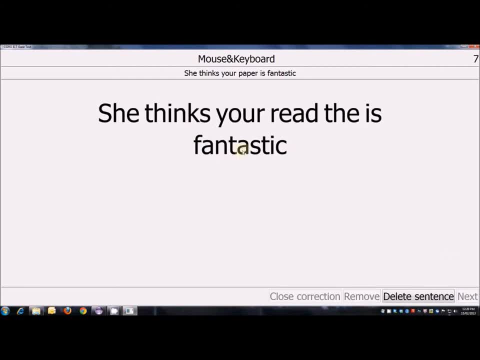 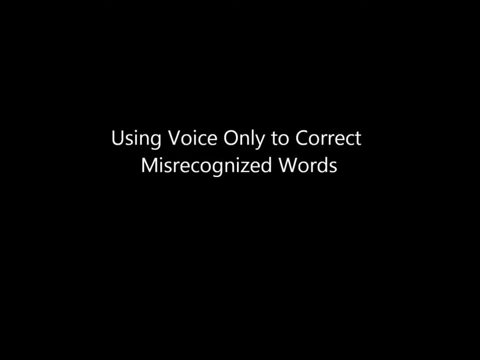 Peter? did you ever think of on the Caramel Island, Peter, when you were young? had you ever thought of the Caramel Island and the American island? Next, we show an example of how to use the voice modality to correct misrecognized words. 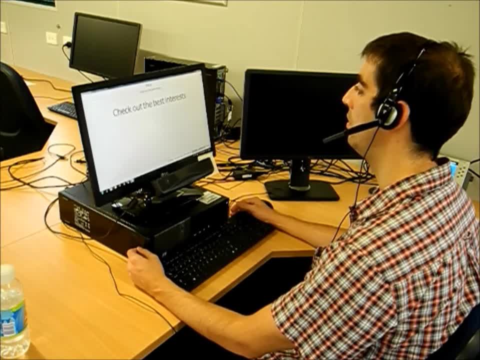 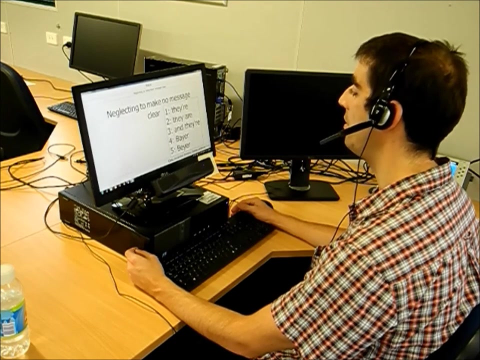 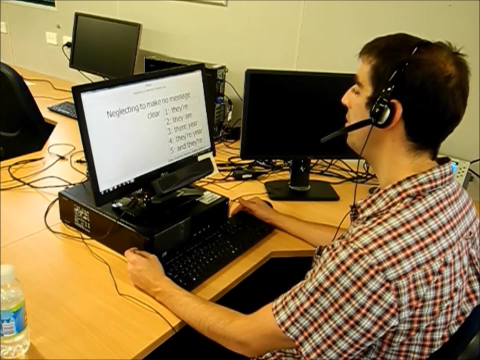 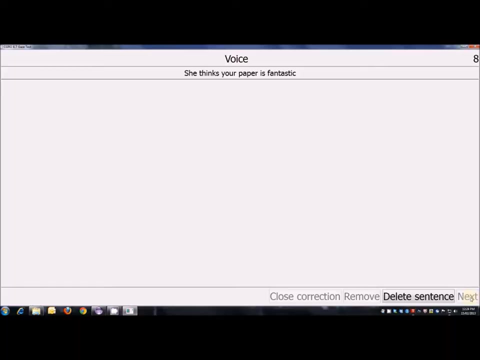 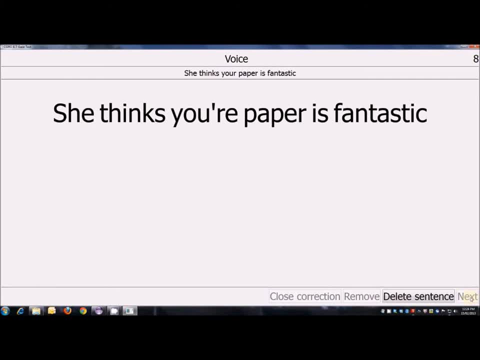 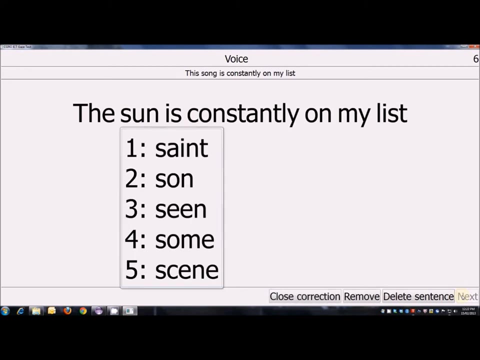 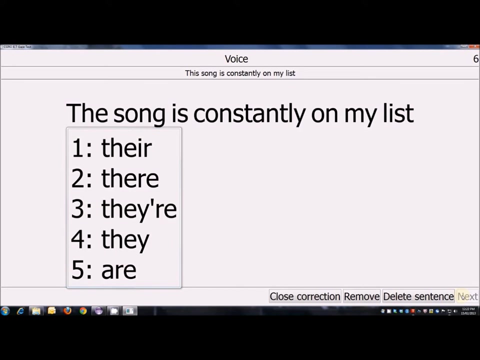 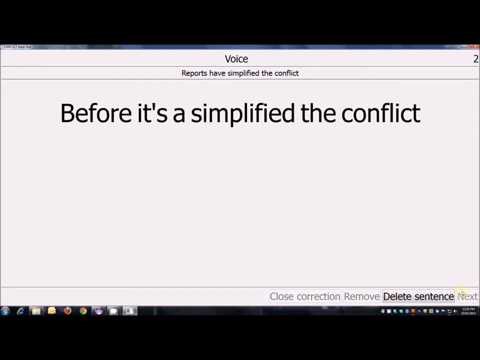 Correct your, Correct you are One. This song is constantly on my list. Correct son Song One. Correct the. This One, This, This. Three Reports have simplified the conflict: Correct before- Correct before Reports. 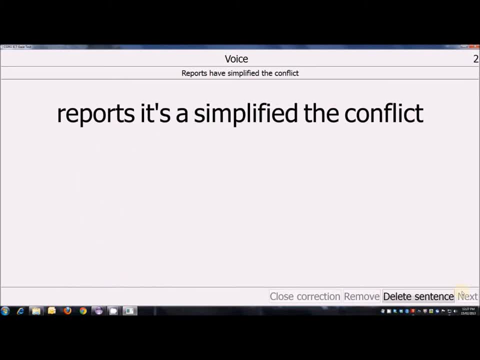 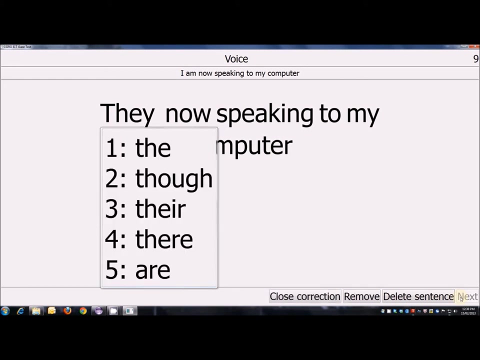 One. it's have to to a remove. I am now speaking to my computer. Correct, no to Correct speaking. Close correction, close correction, Correct they. correct they. Correct they, Correct are. remove, Remove, Correct they, Correct they, I am. 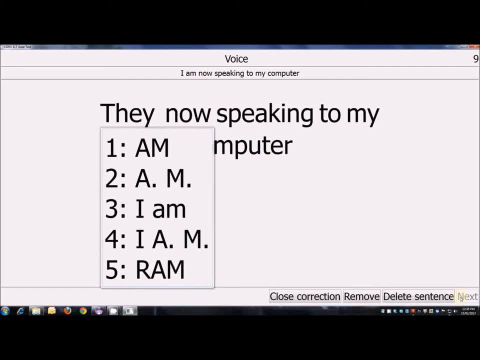 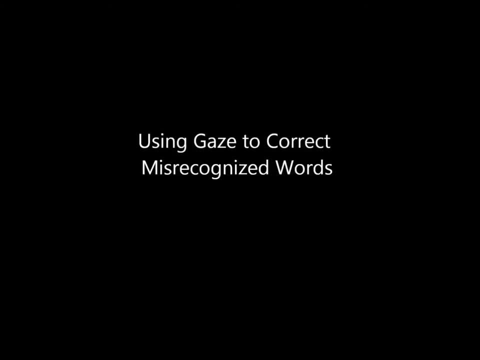 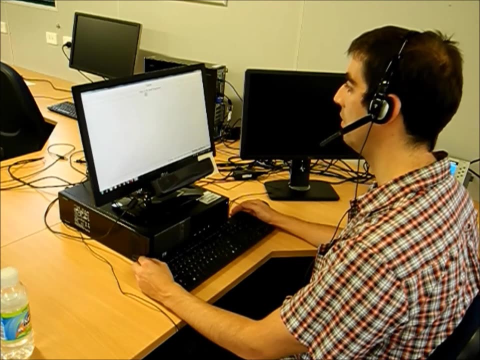 I am Three. And finally, we show an example of how to use gaze to correct misrecognized words. For visualization purposes, we display a subject's gaze as a red disc superimposed over the graphical user interface. This red disc was not visible to subjects during the experimental trials.